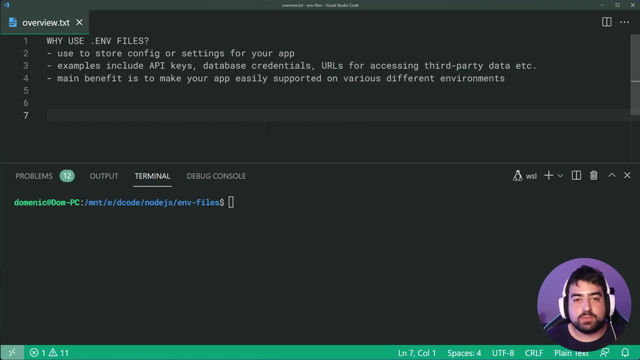 weather application. So your weather application might need something like which country or city to fetch weather for, as well as an API key to actually access the API to retrieve the weather information. So those two things right there, the location and the API key. your friend might have a different API key. 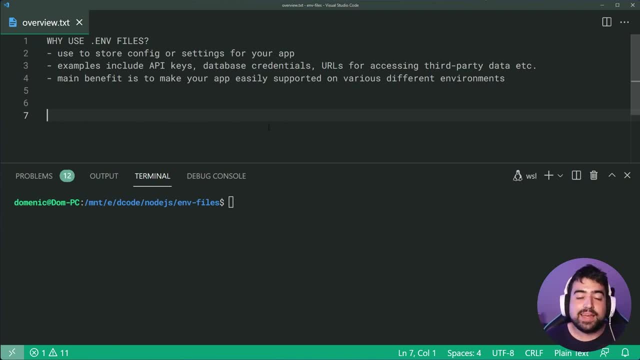 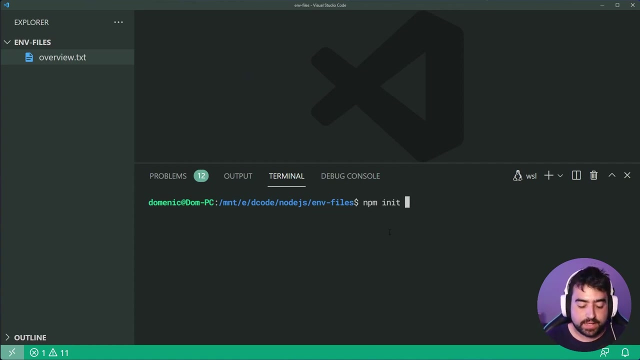 And a different city. therefore, store in the env file and your application will run there perfectly fine. So that is the main motivation behind using a env file. So, when it comes to nodejs, how do you get started in using one? Well, right here I've got a empty directory, so I'm going to make a new nodejs project. I can say npm, init, dash, y and. 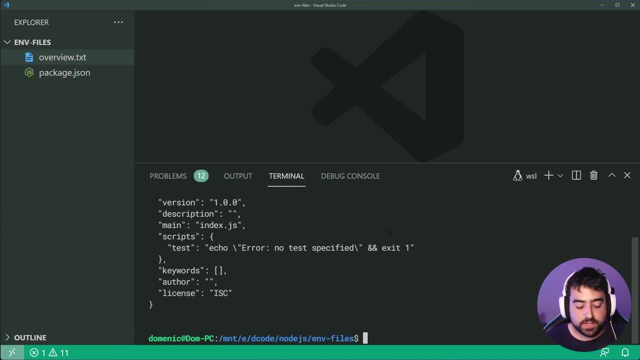 now we have a new nodejs project, So now I just want to install the env file. Okay, so now I've got a new nodejs project. I can say: npm, init, dash, y. and now we have a new nodejs project, so now I just want to install the env file. 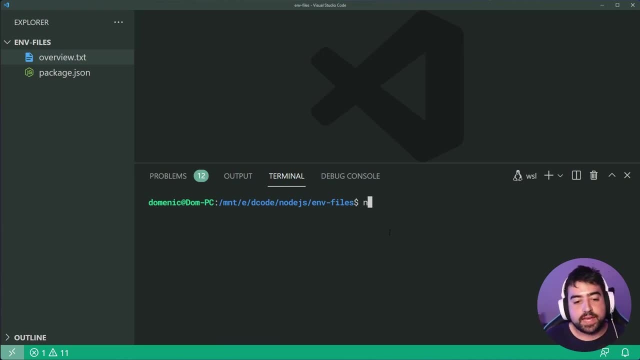 Okay, so now I've got a new nodejs project. I can say npm- init dash y. and now we have a new nodejs project. I can say npm- init dash y. and now we have a new nodejs package. Okay, so right here I'll say npm, i then env, just like that and press enter and of course now it's going to install this nodejs package. 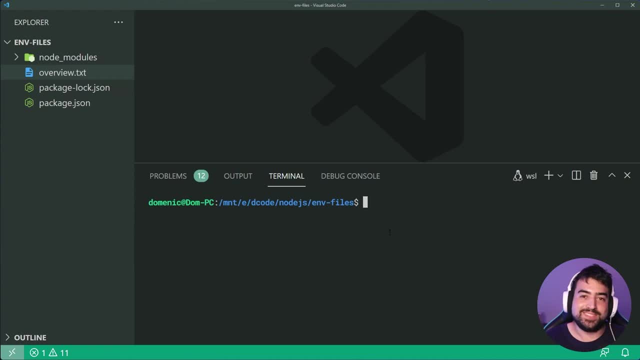 Okay, so now, in order to use, of course, the env package, we're going to need to actually create a env file. So let's make a new file here called env, and then inside here I'm just going to store something like an API key. 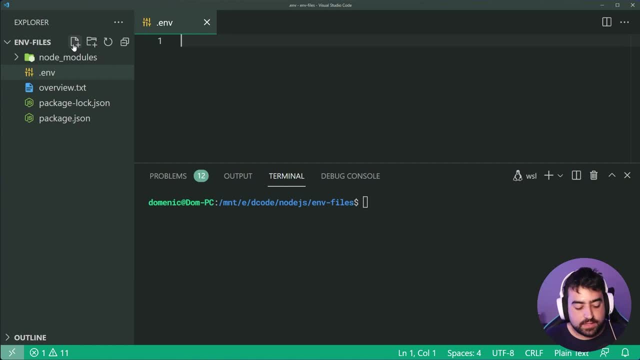 So, going back to the weather example, I can say something like weather API key equal to then 000d32, just as an example. Okay, cool. so right here we have this environmental variable stored inside my env file. So now, how do I access this value in my nodejs application? 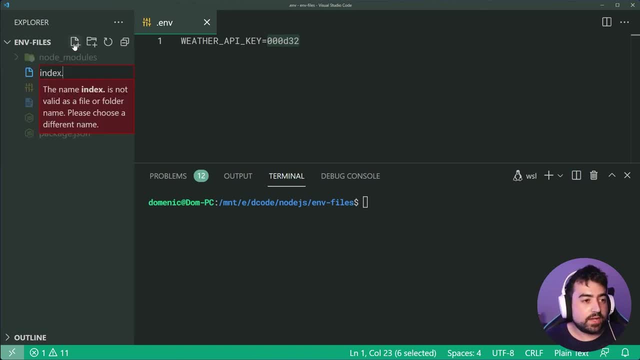 Well, if I make a new indexjs right here and then at the very top I can now require env, but I can actually do it in a bit of a different way. So I can actually just say right here: require just like normal, and then I can say env and then right after it I can say config.